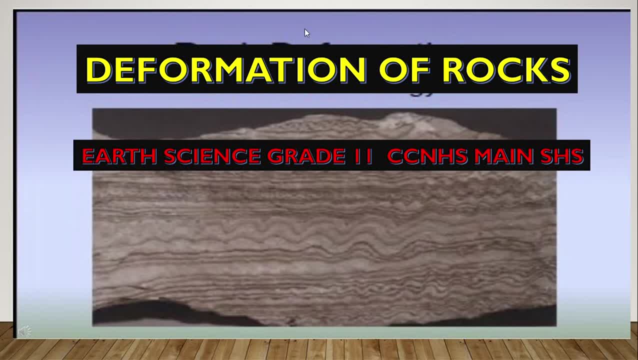 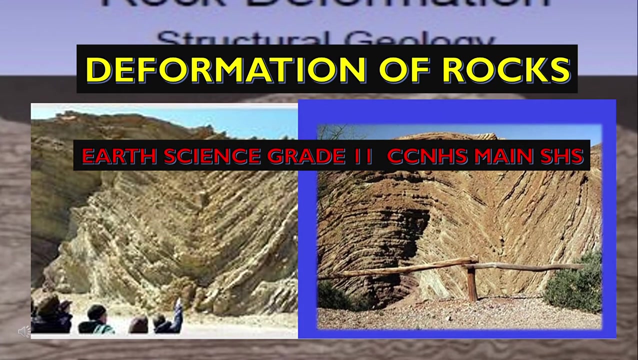 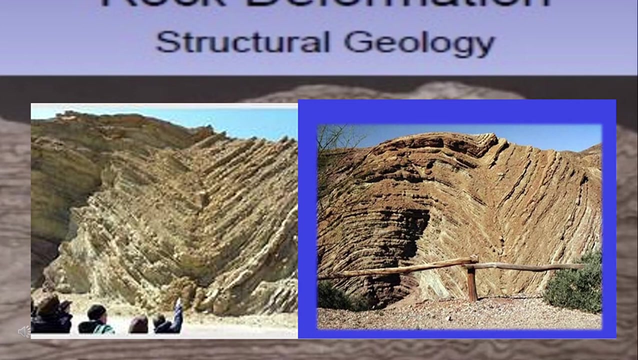 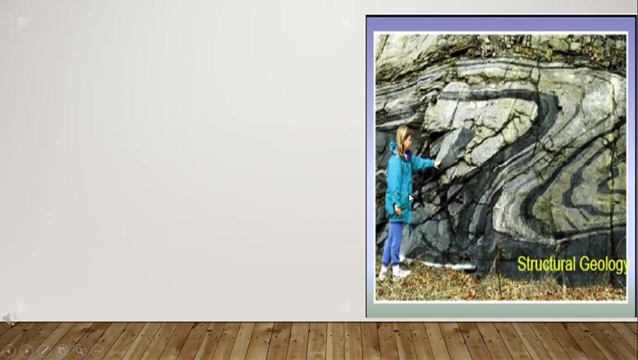 Good morning class. Today we're now on the topic Deformation of Racks. This is the Earth Science of Grade 11 of Kaua'i City National High School, Maine Senior High School. So how the racks are being deformed. 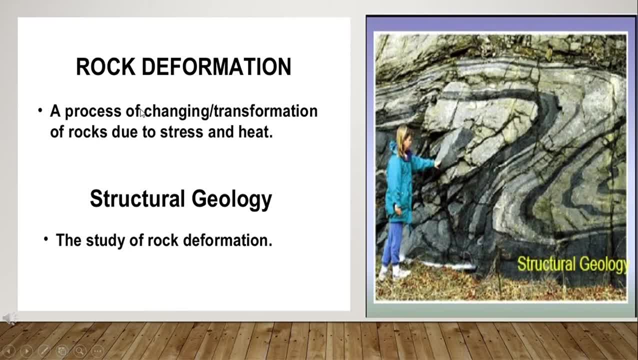 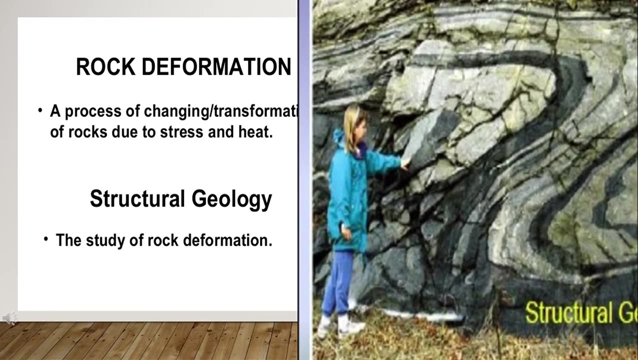 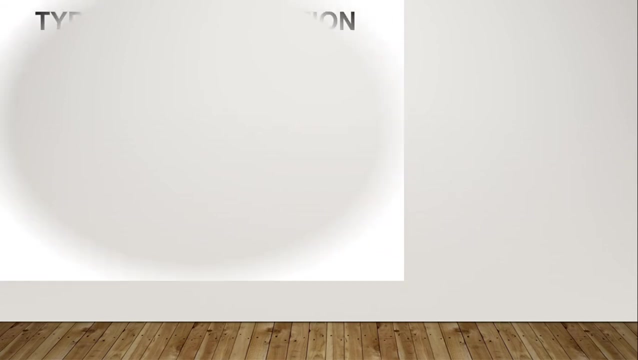 Rack deformation is a process of changing transformation of racks due to stress and heat. Structural geology is the study of rack deformation. There are types of deformation of racks. Number one is faults, the second is faults and the third one is joints. 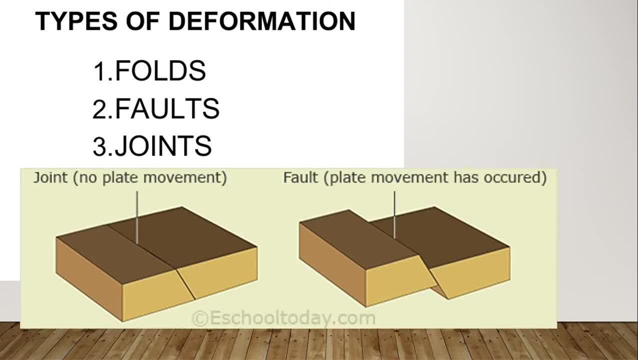 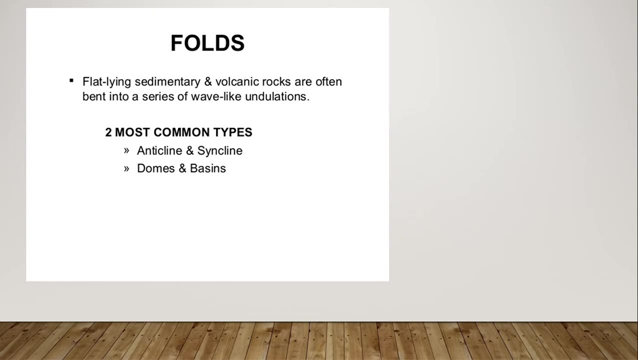 Joint has no plate movement. Fault has plate movement that has occurred. Faults are flat lying sedimentary rocks. Faults are flat lying sedimentary and volcanic rocks that are often bent into a series of wave-like indulations. There are two most common types: the anticline and the syncline domes and basins. 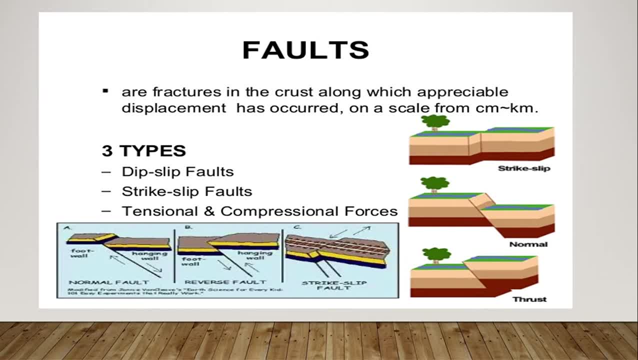 Faults. Faults are fractures in the crust along which appreciable displacement has occurred, on a scale from centimeter to kilometer. There are three types of faults: One is deep slip faults, The other one is strike slip faults And the third one is the tensional and compressional. 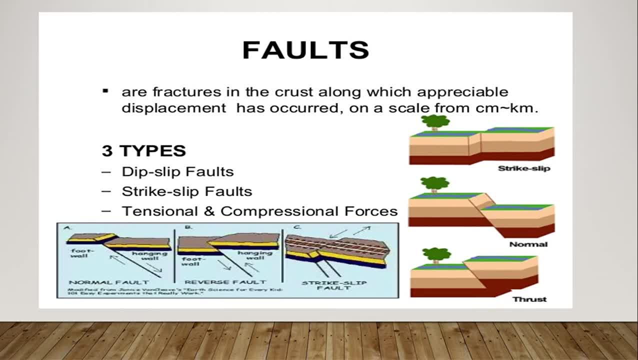 forces faults, which is the truss. This is the strike slip That is slip'd for a little bit distance, And this is the normal faults. And this is the truss too, The normal faults. One is going up on the left side. 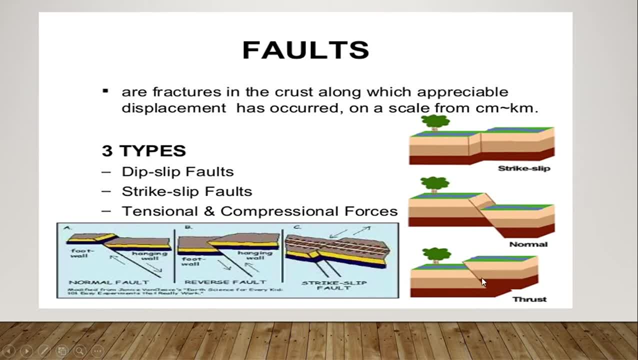 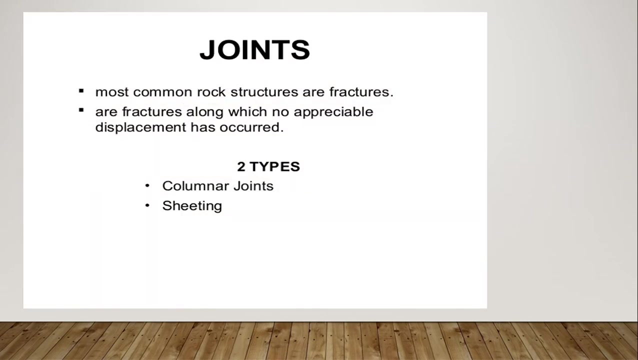 and the other one is going up down to the right side, while the trust is the opposite of the normal. the other one is going to going the right one, the right side is going up and the left side is going down. that is false. what about joints? joints are most common. 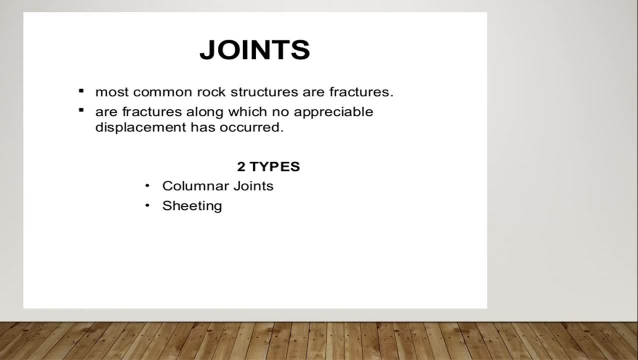 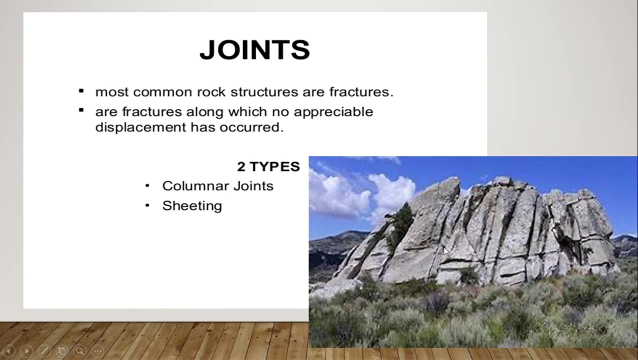 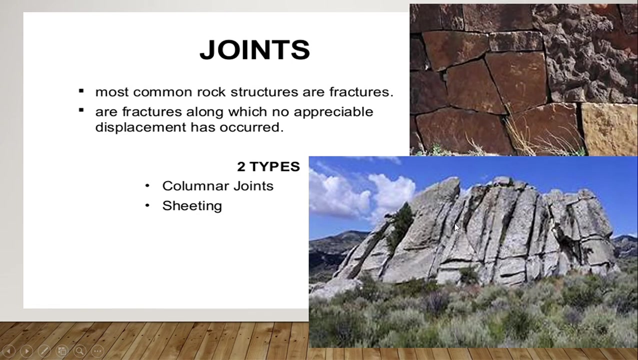 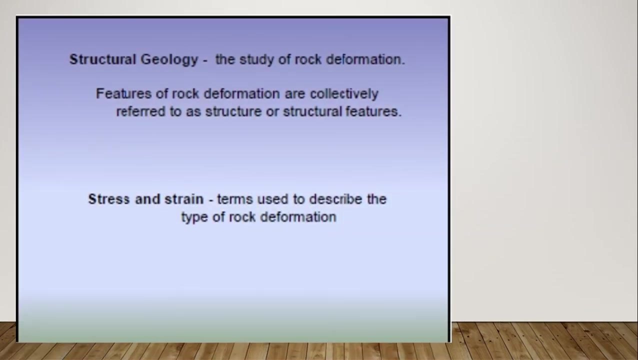 rock structures which are fractures. these are fractures along which new appreciable displacement has occurred. there are two types of joints: one is columnar joints and the other one is heating joints. so this is how a joint looks like. there are fractures between the racks. structural geology is the study of rock deformation. features of rock deformation. 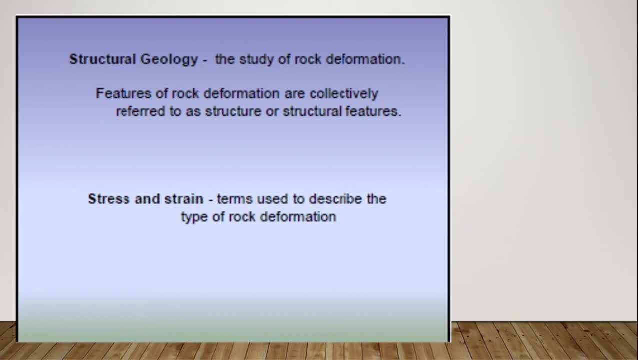 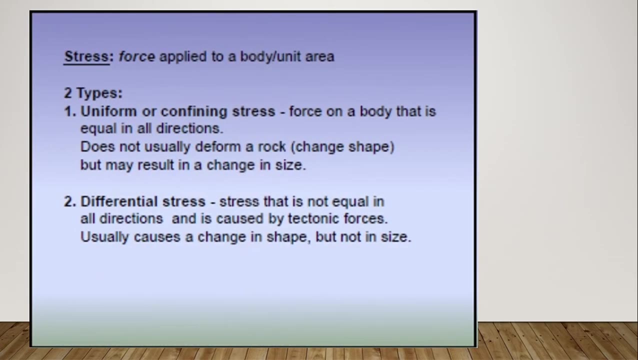 are collectively referred to as structure or structural features, stress and strain terms. these are used to describe the type of rock deformation. stress is the force applied to a body. stress is the force applied to a body. stress is the force applied to a body or a unit area. there are two types of 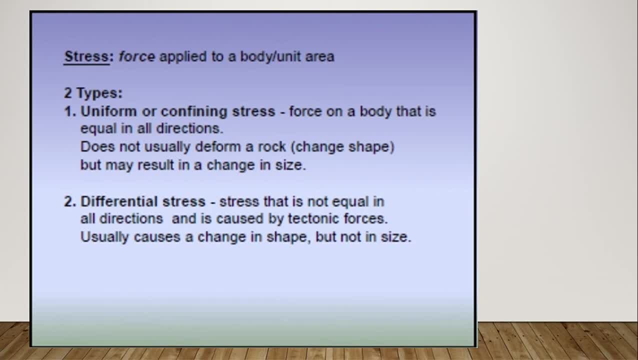 or a unit area. there are two types of or a unit area. there are two types of stress. one is uniform or confining stress. one is uniform or confining stress. one is uniform or confining stress, which is the portion of body that stress, which is the portion of body that 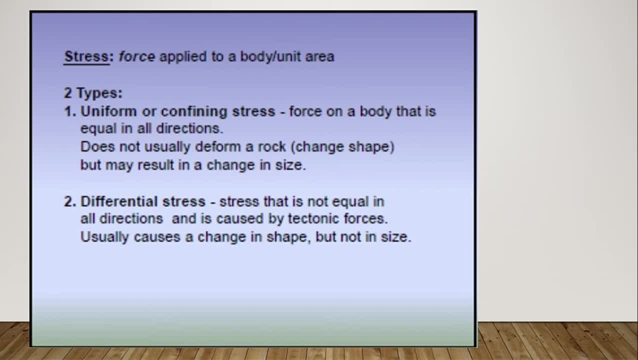 stress, which is the portion of body that is equal in all directions. does not is equal in all directions. does not is equal in all directions. does not usually deform a rack or a change the usually deform a rack or a change. the usually deform a rack or a change the rack shape, but may result in a change in. 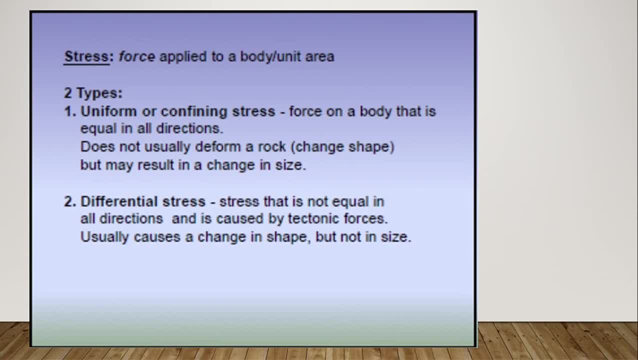 rack shape but may result in a change in rack shape, but may result in a change in the size of the rock. the other one is the size of the rock. the other one is the size of the rock, the other one is differential stress. these are stress that 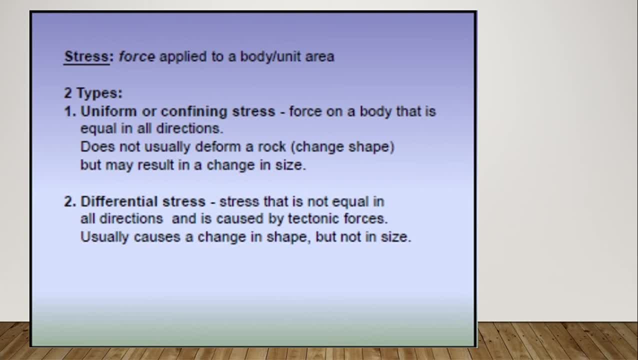 differential stress. these are stress, that differential stress. these are stress that is not equal in all directions and is is not equal in all directions and is is not equal in all directions and is caused by tectonic forces usually causes. caused by tectonic forces usually causes. 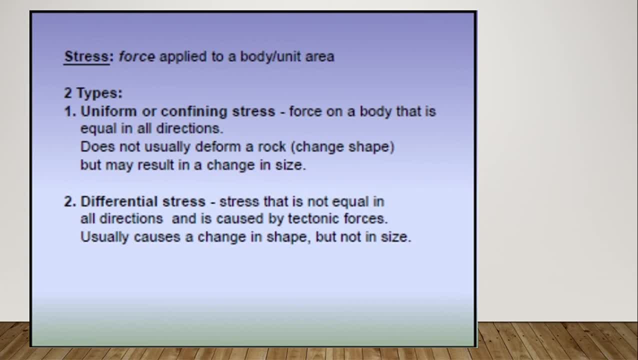 caused by tectonic forces usually causes us change in shape but not in size. so us change in shape but not in size. so us change in shape but not in size. so the opposite of uniform confining stress, the opposite of uniform confining stress, the opposite of uniform confining stress, is differential stress. there are three. 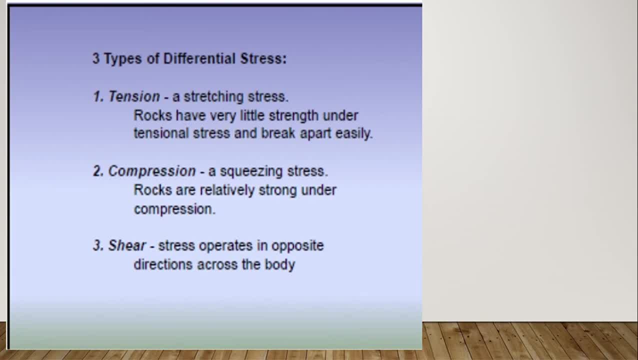 is differential stress. there are three is differential stress. there are three types of differential stress. one is types of differential stress. one is types of differential stress. one is tension, which is a stretching stress. tension which is a stretching stress. tension which is a stretching stress, where in rocks have very little. 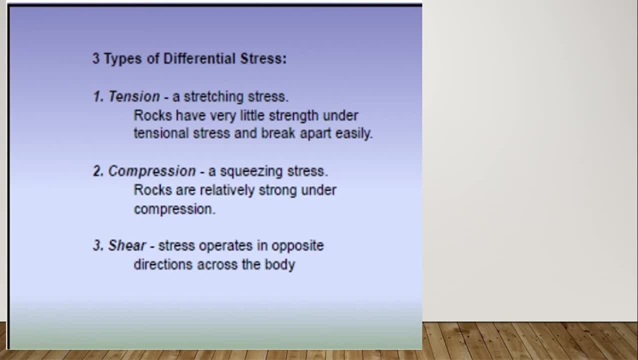 where in rocks have very little, where in rocks have very little strength and their attention on stress strength and their attention on stress strength and their attention on stress and break apart easily. the second one is: and break apart easily. the second one is: and break apart easily. the second one is compression. it is the squeezing stress. 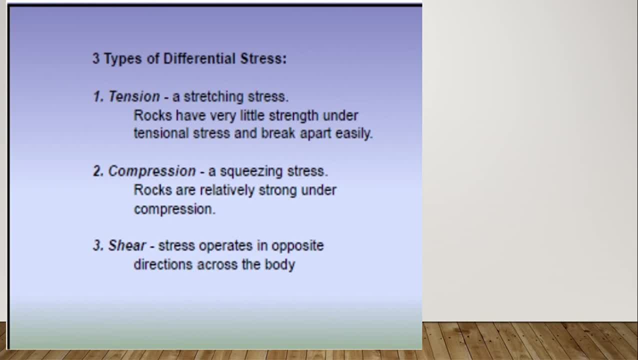 compression. it is the squeezing stress compression. it is the squeezing stress. rocks are ready to be strong under this. rocks are ready to be strong under this. rocks are ready to be strong under this compression. the third one is the shear compression. the third one is the shear compression. the third one is the shear stress operates in opposite direction. 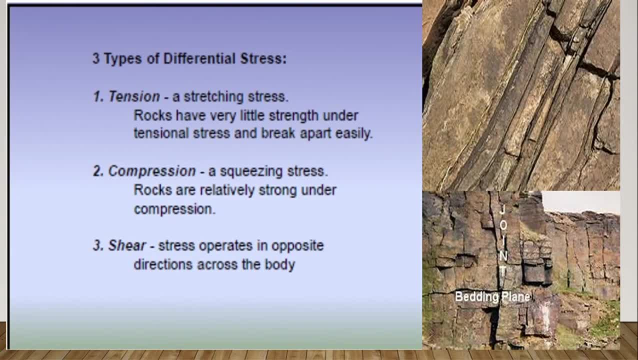 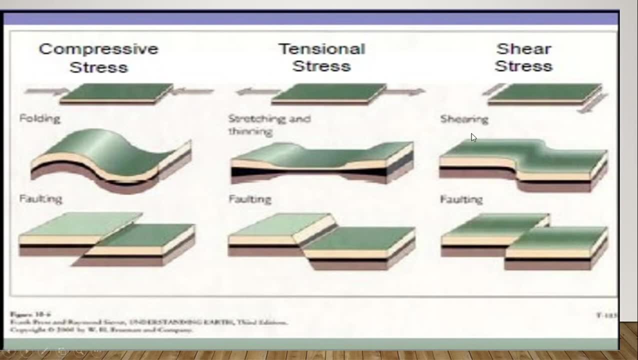 stress operates in opposite direction. stress operates in opposite direction, across the body. so this is the across the body, so this is the across the body. so this is the compressive stress, the tension of stress, compressive stress, the tension of stress, compressive stress, the tension of stress and the shear stress. 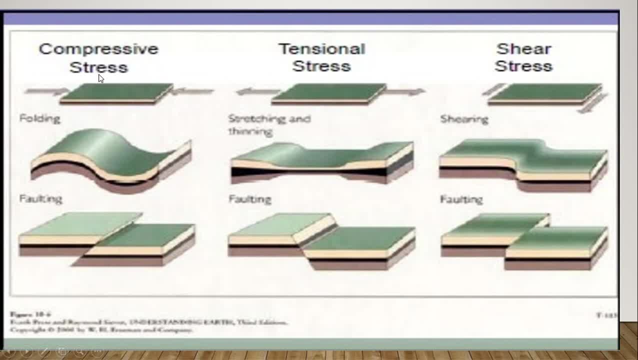 and the shear stress and the shear stress. so when under compressive stress, so when under compressive stress, so when under compressive stress, folding is like this, so compressive folding is like this, so compressive folding is like this. so compressive stress, it was the rocks and it results to 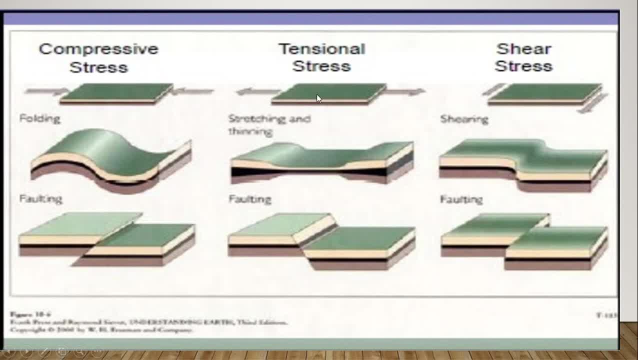 stress it was the rocks and it results to stress it was the rocks and it results to faulting national stress. results to faulting national stress. results to faulting national stress. results to stretching and cleaning of the rocks and stretching and cleaning of the rocks and stretching and cleaning of the rocks and also faulting shear stress results. 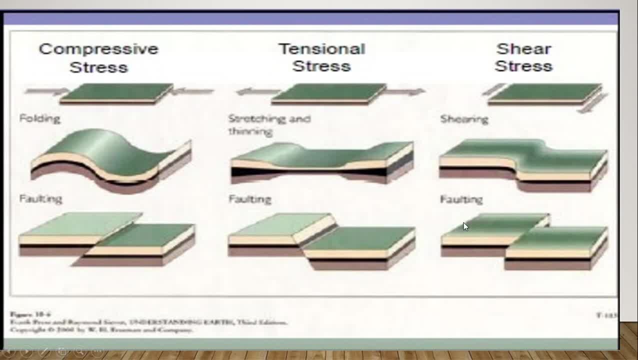 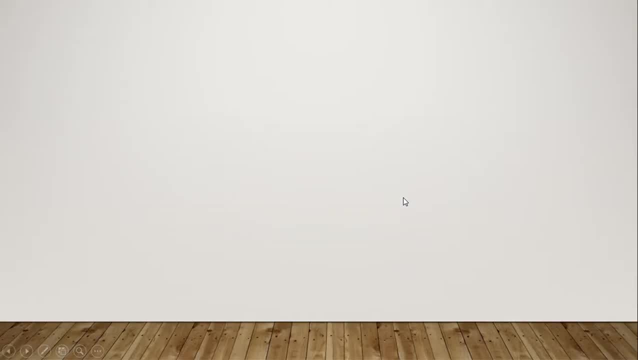 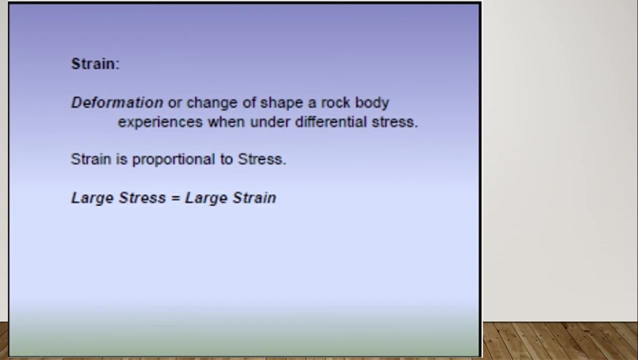 also faulting shear stress results also faulting shear stress results in shearing and it also results to in shearing and it also results to in shearing and it also results to faulty strain. strain is the deformation. faulty strain. strain is the deformation. faulty strain strain is the deformation or change of shape of a rock body. 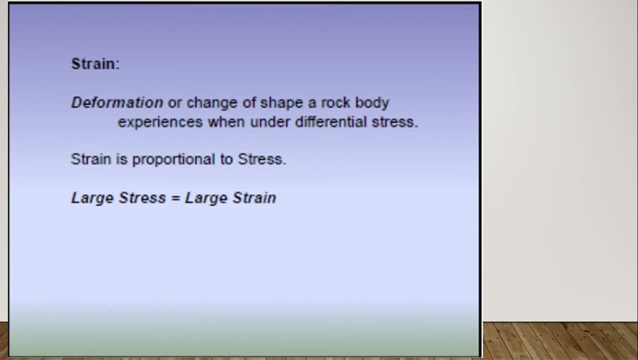 or change of shape of a rock body or change of shape of a rock body. experience has been under differential. experience has been under differential. experience has been under differential. stress strain is proportional to stress. stress strain is proportional to stress. stress strain is proportional to stress, so large stress is equal to large. 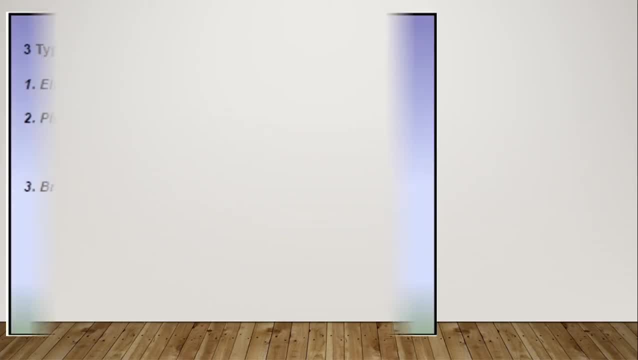 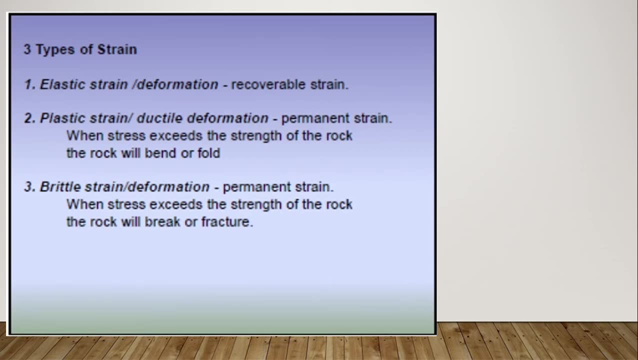 so large stress is equal to large, so large stress is equal to large strains, strains, strains. there are three types of strain. one is: there are three types of strain. one is: there are three types of strain. one is elastic strain deformation, which is elastic strain deformation, which is: 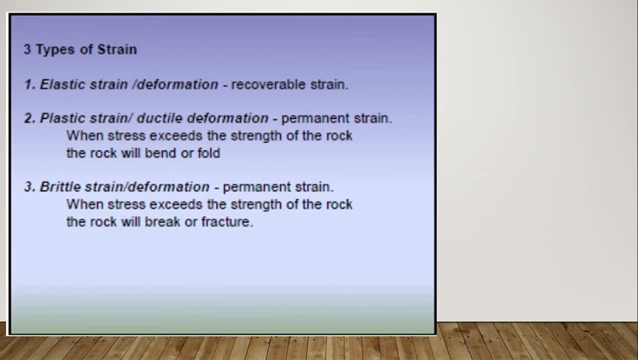 elastic strain deformation, which is recoverable strain. the second one is recoverable strain. the second one is recoverable strain. the second one is plastic strain ductile deformation, which plastic strain ductile deformation, which plastic strain ductile deformation, which is a permanent strain when stress, is a permanent strain when stress. 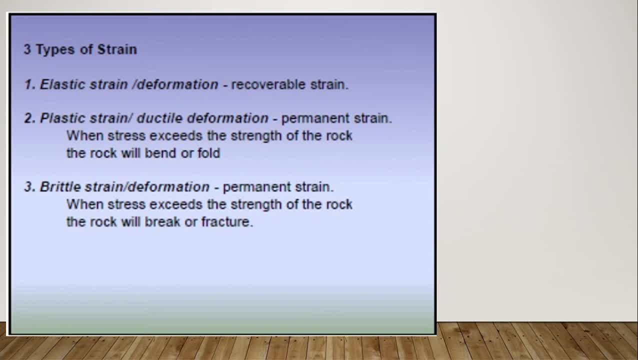 is a permanent strain when stress exceeds the strength of the rock. the exceeds the strength of the rock. the exceeds the strength of the rock. the rock will bend or fold. the third one is: rock will bend or fold. the third one is: rock will bend or fold. the third one is brittle strain: deformation. it is a. 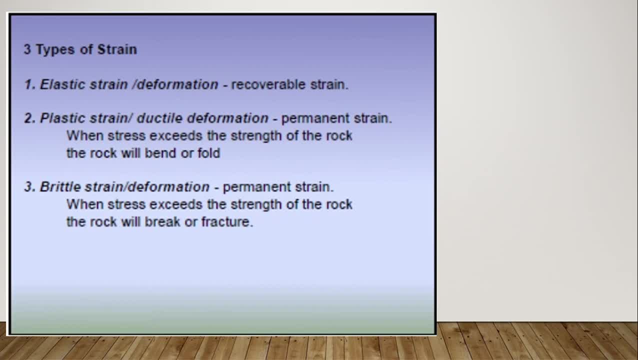 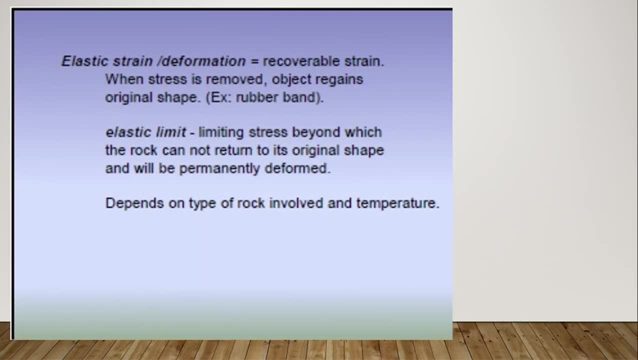 brittle strain deformation. it is a brittle strain deformation. it is a permanent strain when stress exists. the permanent strain when stress exists. the permanent strain when stress exists. the strength of the wrap: the rack will break. strength of the wrap: the rack will break. strength of the wrap: the rack will break or fracture. less extreme deformation is 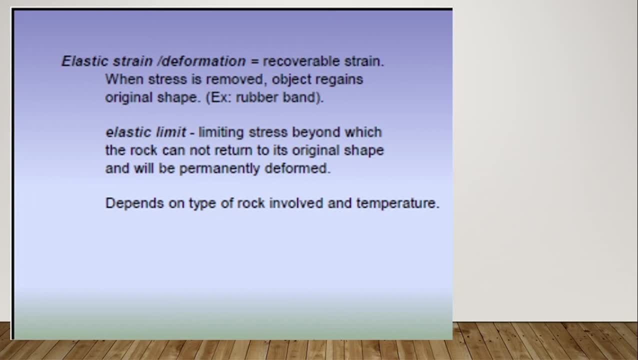 or fracture less extreme deformation is, or fracture less extreme deformation is the recoverable strain when stress is the recoverable strain. when stress is the recoverable strain when stress is removed. object regains original shape removed. object regains original shape removed. object regains original shape like a rubber band. elastic limit is the. 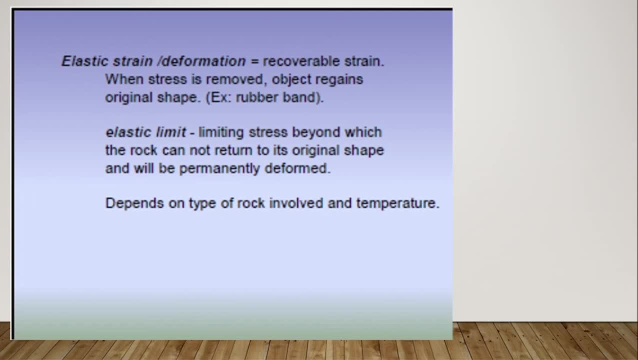 like a rubber band elastic limit is the like a rubber band. elastic limit is the limiting stress beyond which the rack limiting stress beyond which the rack- limiting stress beyond which the rack cannot return to its original shape and cannot return to its original shape and cannot return to its original shape and will be permanently deformed- depends on. 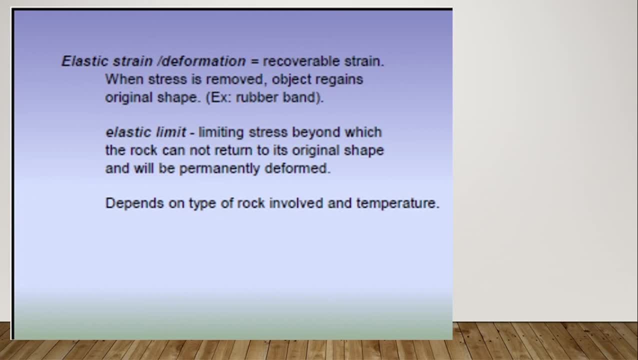 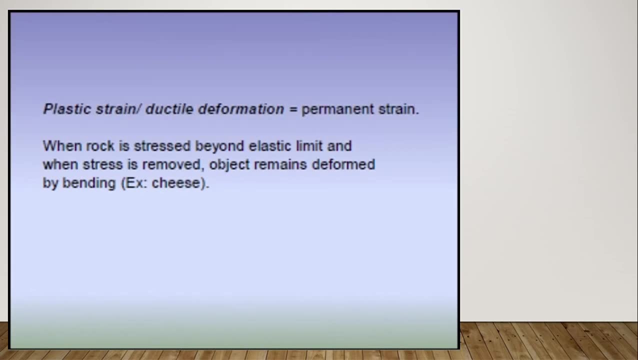 will be permanently deformed. depends on: will be permanently deformed. depends on the wrap. it will end the wrap. it will end the wrap. it will end temperature or the wrap type and the temperature. or the wrap type and the temperature. or the wrap type and the temperature. 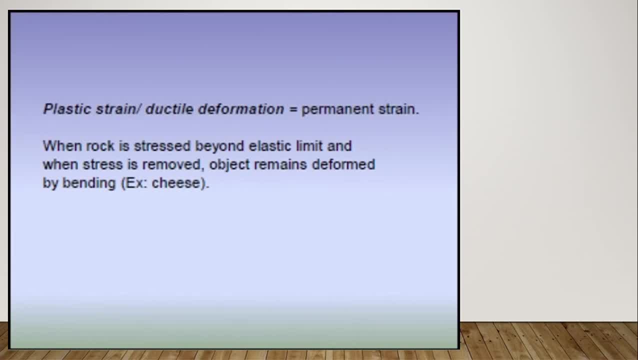 plastic strain ductile deformation. which plastic strain ductile deformation, which plastic strain ductile deformation, which is a permanent strain, is a permanent strain, is a permanent strain. happens when rack is stressed beyond. happens when rack is stressed beyond. happens when rack is stressed beyond elastic limit and when stress is removed. 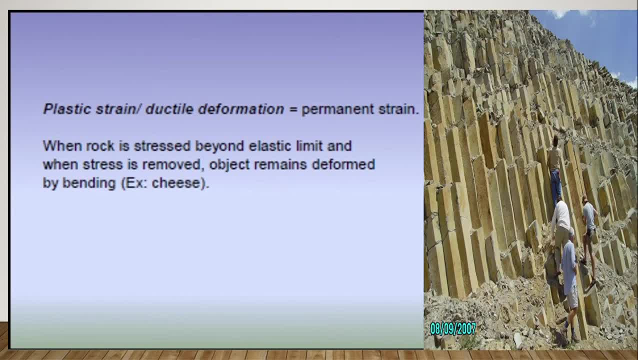 elastic limit and when stress is removed. elastic limit and when stress is removed, the object remains deformed. by bending: the object remains deformed by bending. the object remains deformed by bending, for example, like cheese. little strain deformation, it is a little strain deformation, it is a 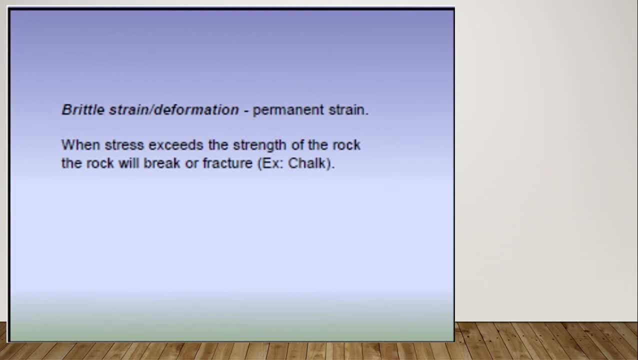 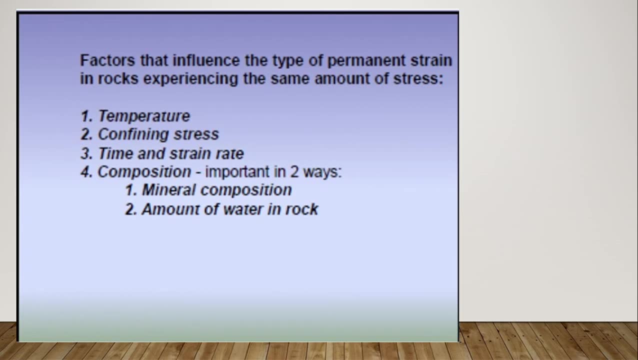 little strain deformation. it is a permanent strain. permanent strain. permanent strain when stress exceeds the strength of the wrap. when stress exceeds the strength of the wrap. when stress exceeds the strength of the wrap, the rack will break or fracture. for the rack will break or fracture. for the rack will break or fracture, for example, shock factors that influence the 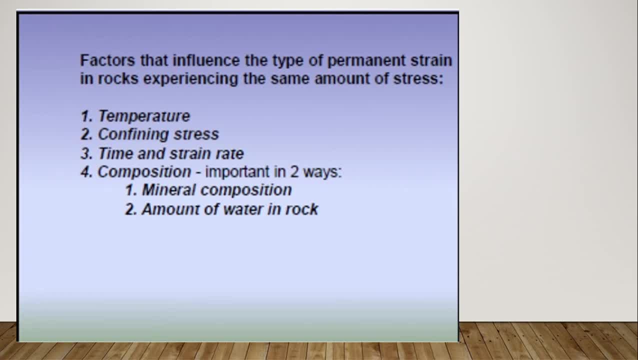 example, shock factors that influence the example. shock factors that influence the type of permanent strain in grass, type of permanent strain in grass, type of permanent strain in grass, experiencing the same amount of stress, experiencing the same amount of stress, experiencing the same amount of stress. we have number one: the temperature. 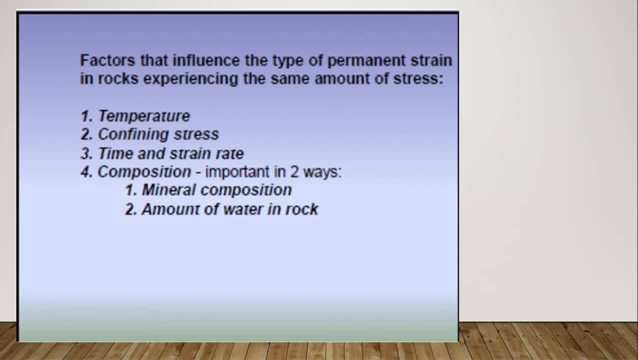 we have number one, the temperature. we have number one, the temperature. second one confining stress. third time: second one, confining stress, third time. second one, confining stress, third time, and strain rate. the fourth one is and strain rate. the fourth one is and strain rate, the fourth one is competition, important in two ways. one, it 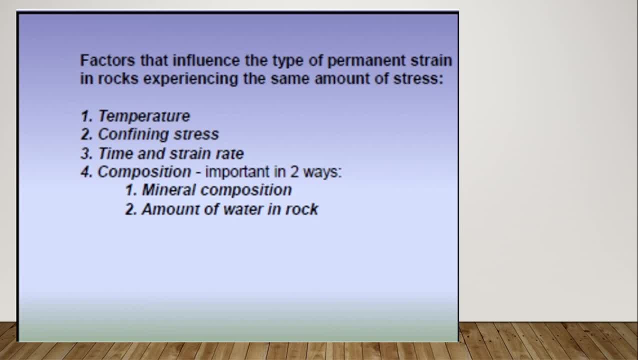 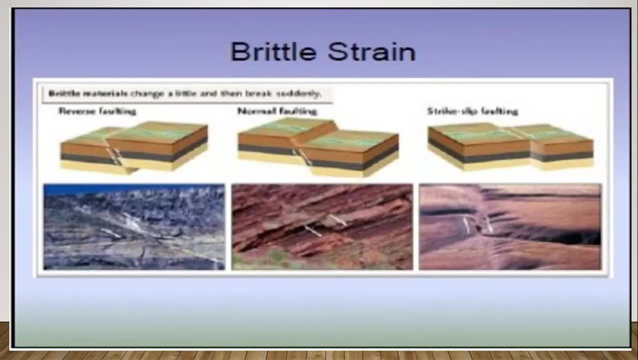 competition important in two ways. one: it competition important in two ways. one, it is important in mineral composition and is important in mineral composition and is important in mineral composition. and second, one is the amount of water in second. one is the amount of water in second. one is the amount of water in rack. so this is how the result strain. 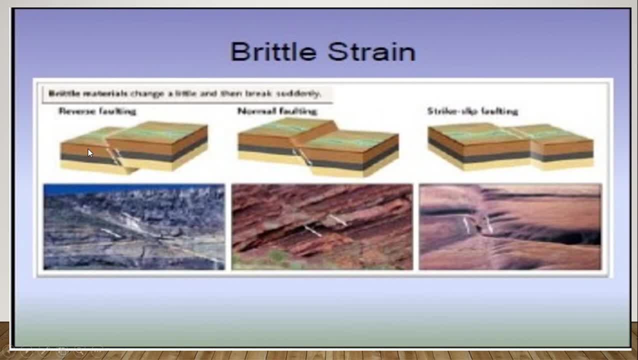 rack. so this is how the result strain rack. so this is how the result strain: looks nice. it results to the reverse: looks nice. it results to the reverse: looks nice. it results to the reverse, faulting the normal faulting and the faulting the normal faulting and the. 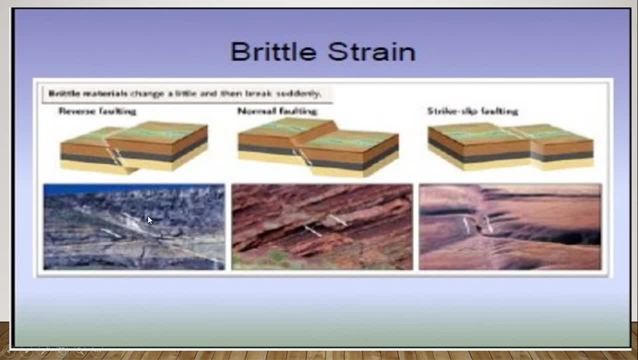 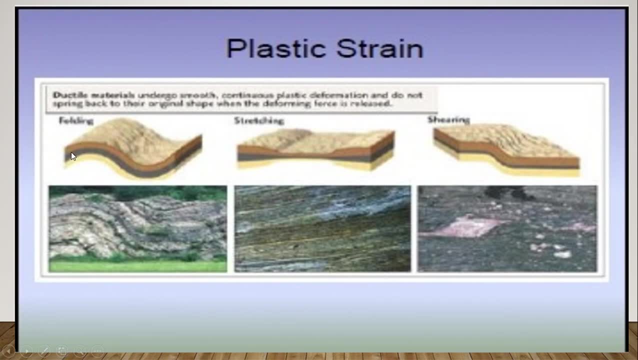 faulting, the normal faulting and the strike sleep faulting looks like this strike sleep faulting. looks like this strike sleep faulting. looks like this plastic strain, plastic strain, plastic strain. it will not still result fully 18 straight. it will not still result fully 18 straight. 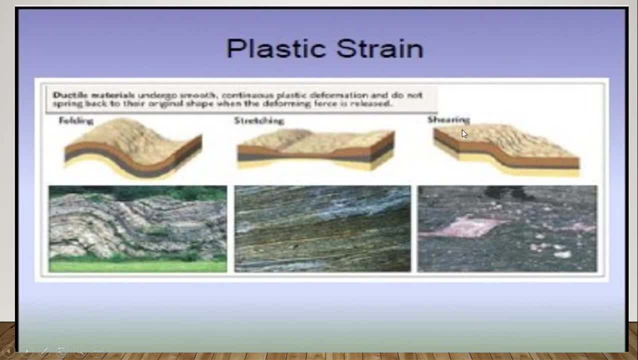 it will not still result fully. 18 straight unfolding, stretching and shearing. this unfolding, stretching and shearing. this unfolding, stretching and shearing. this is folding stretching. this is hearing. is folding stretching. this is hearing. is folding stretching. this is hearing. plastic strain: folding is the horizontal. 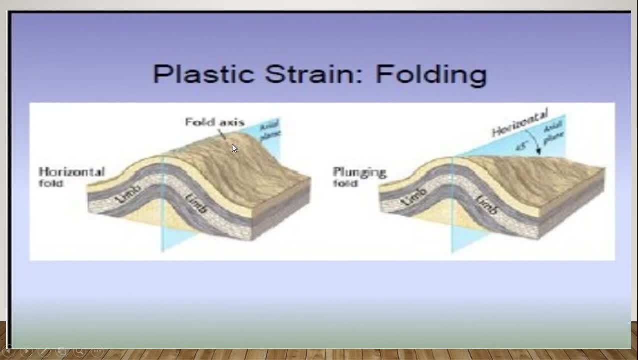 plastic strain folding is the horizontal plastic strain folding is the horizontal fold, the fold of axis when strain is fold. the fold of axis when strain is fold, the fold of axis when strain is being applied, being applied, being applied, it will form like this: the rock will. it will form like this: the rock will. 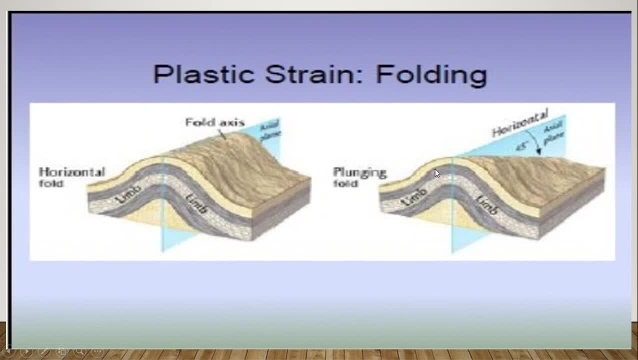 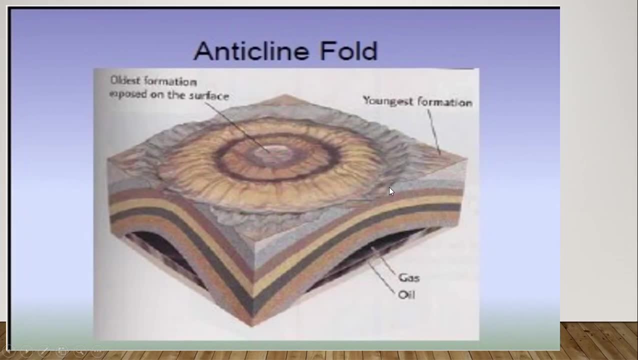 it will form like this. the rock will form like this. this is the flying fold form like this. this is the flying fold form like this. this is the flying fold. this is the horizontal axis. the. this is the horizontal axis, the. this is the horizontal axis. the anticline fold, the oldest formation. 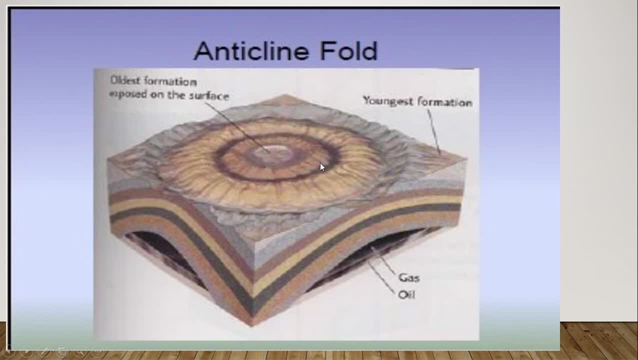 anticline fold, the oldest formation. anticline fold, the oldest formation exposed on the surface. this is the exposed on the surface. this is the exposed on the surface. this is the youngest formation and this is youngest formation and this is youngest formation. and this is the buzzer guys and oil. this is an. 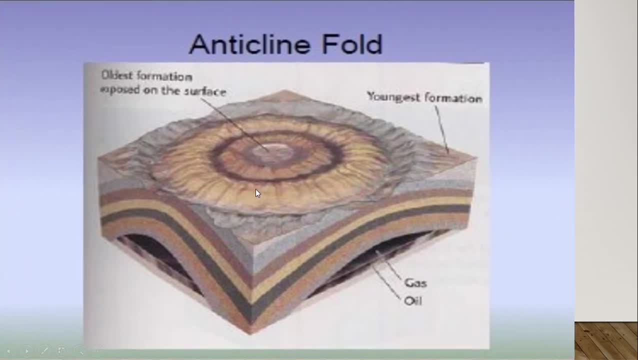 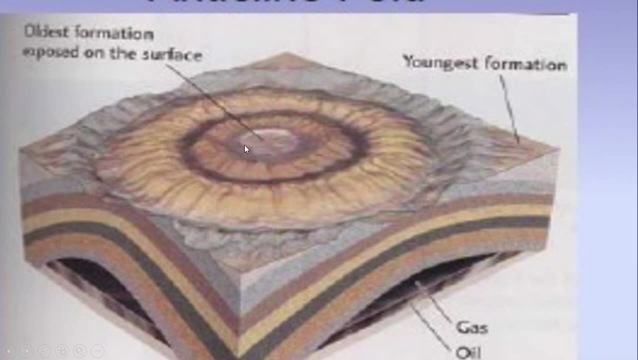 the buzzer guys and oil. this is an the buzzer guys and oil. this is an anti-client, anti-client, anti-client, anti-client, anti-client, anti-client, anti-client fault. you can see here the oldest formation fault. you can see here the oldest formation fault. you can see here the oldest formation exposed of the surface, the 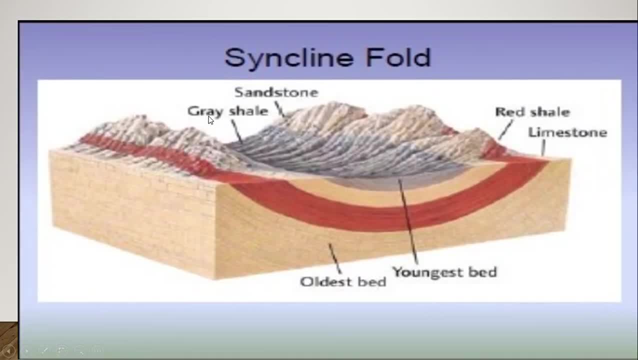 exposed of the surface. the exposed of the surface. the inclined fold. we have the sandstone inclined fold. we have the sandstone inclined fold. we have the sandstone. the gray tail. the red airline is the? the gray tail. the red airline is the? the gray tail. the red airline is the bus line stone. this is the youngest. 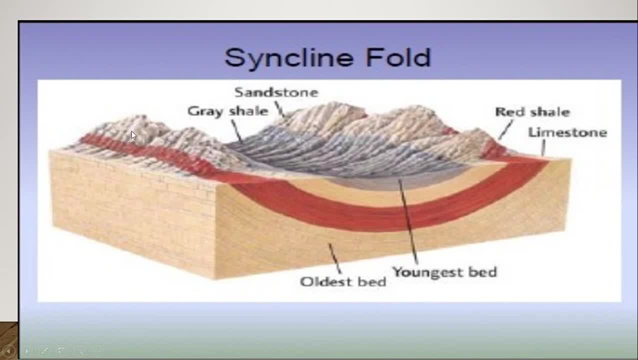 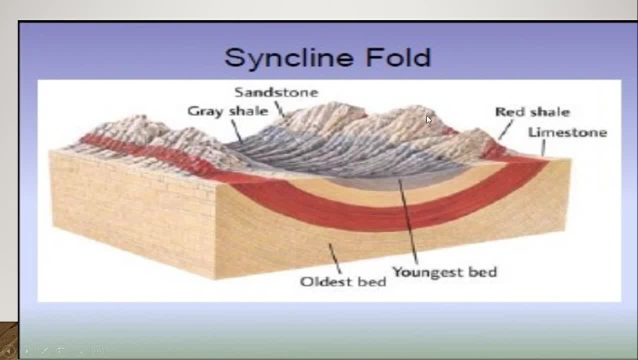 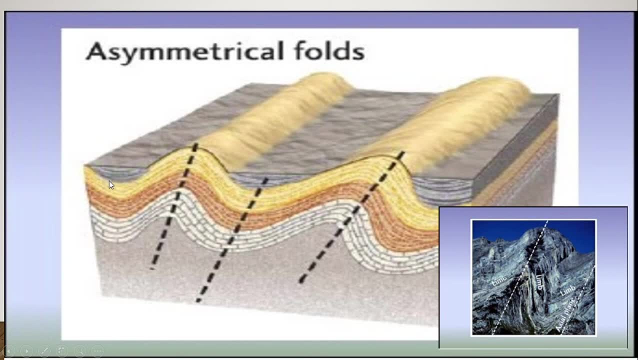 looks like we have the upper surface here. looks like we have the upper surface here. and it comes from different types of, and it comes from different types of and it comes from different types of rocks asymmetrical fold looks like this. rocks asymmetrical fold looks like this. 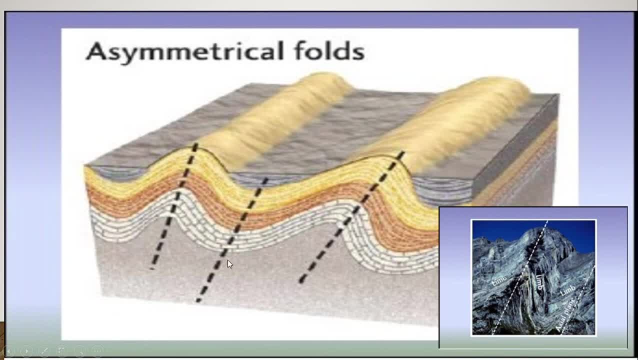 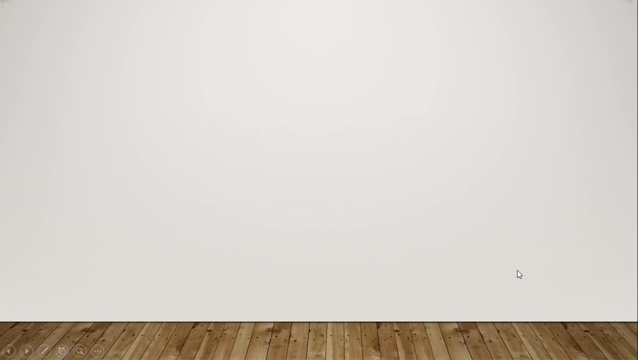 rocks asymmetrical fold looks like this: the direction is upward and it warms. the direction is upward and it warms. the direction is upward and it warms like a wave like this one over, like a wave like this one over, like a wave like this one over june. 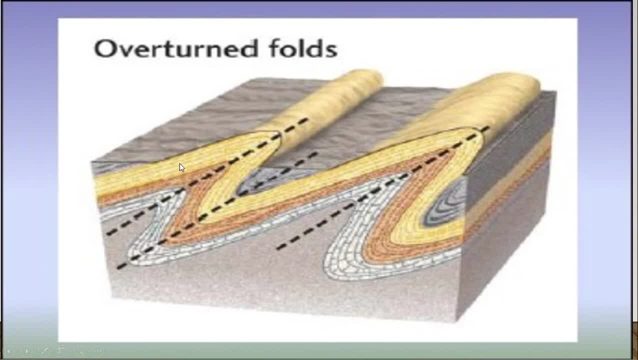 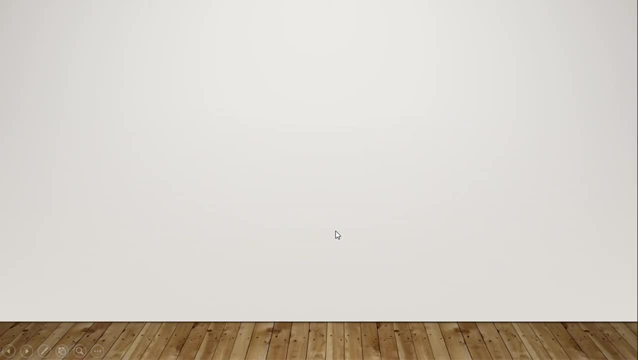 june, june. falls: this is a more bent or more ways. falls. this is a more bent or more ways. falls. this is a more bent or more ways. bending to the right side direction. bending to the right side direction. bending to the right side direction. flying force: this is how. flying holes. 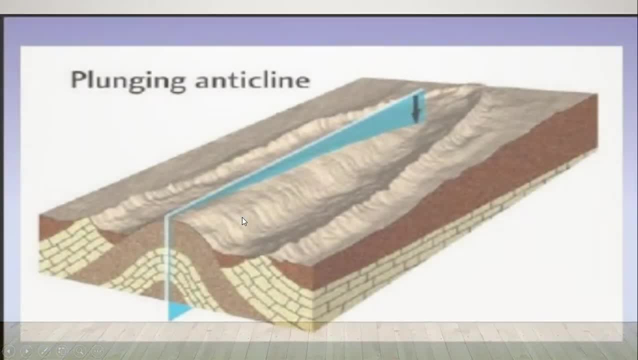 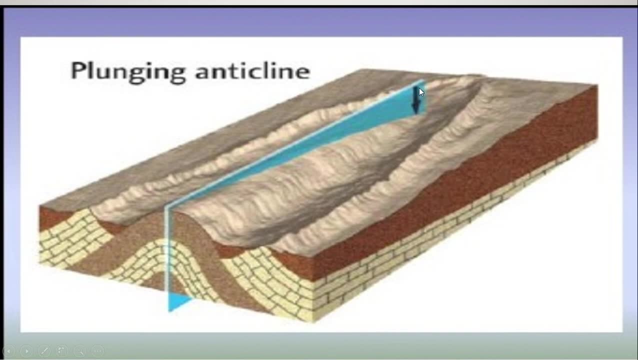 flying force. this is how flying holes flying force. this is how flying holes looks like. flying and decline. you can looks like flying and decline. you can looks like flying and decline. you can see some falls when there is a flying. see some falls when there is a flying. 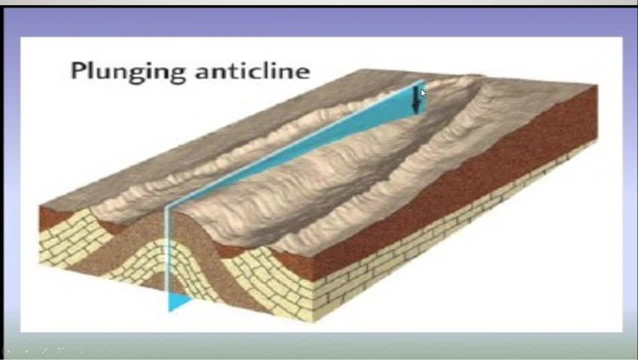 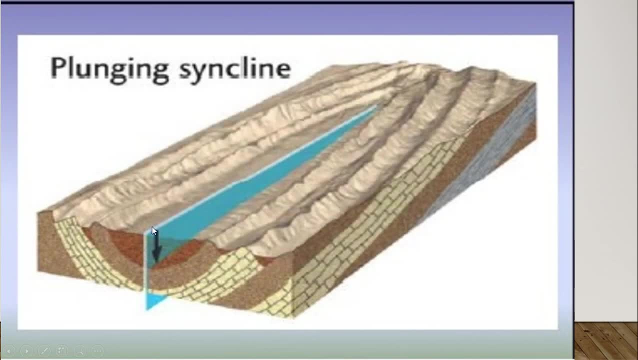 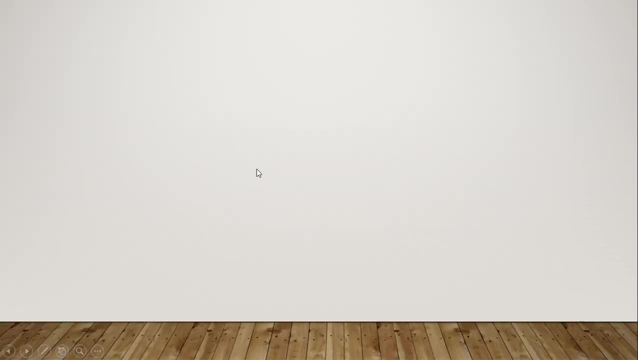